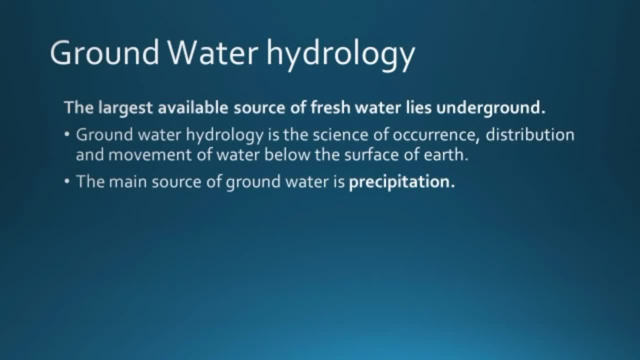 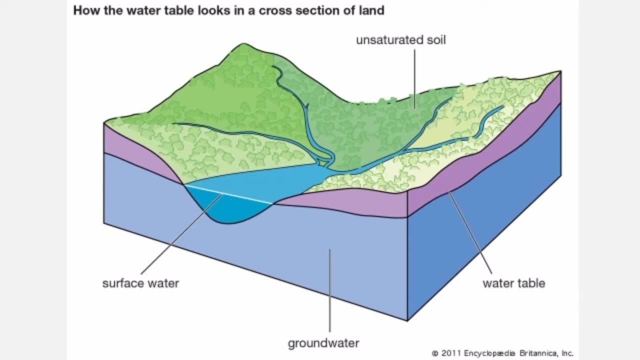 reaching the groundwater below water table. That is the main source. So, for better understanding, this is groundwater, The line that separates that purple part, which is the unsaturated soil, and the blue part, which is the groundwater or saturated soil. So the blue part, which is the unsaturated 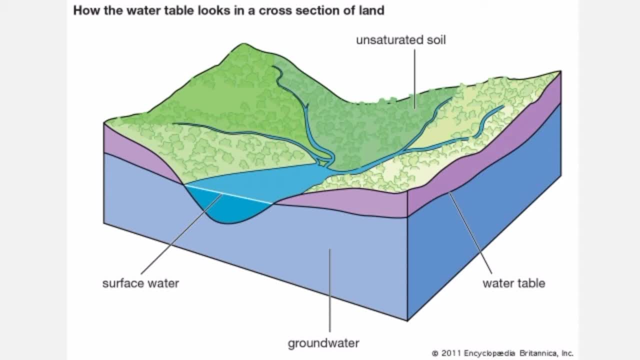 soil is called water table, and surface water is what we normally called as lakes, oceans, seas, ponds, rivers, etc. that we can see and observe from the surface itself. and groundwater is what we are concerned of now, So that blue part, or the groundwater or saturated soil part, can be soil, rock, clay or many. 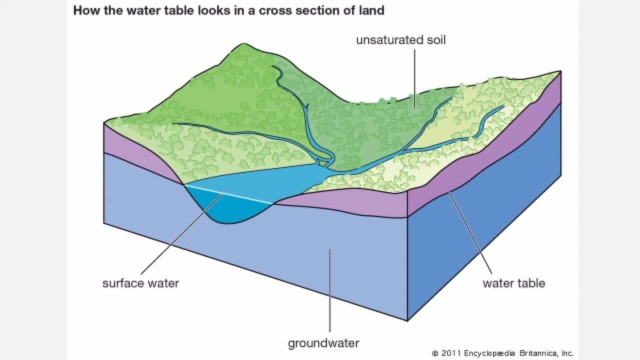 variations. we call it as formations. This formations will vary place to place. In some places it will be clay formation. in some places it will be sandy, it will be gravel formations, some in some places it will be rocky formations. So based on that, we have 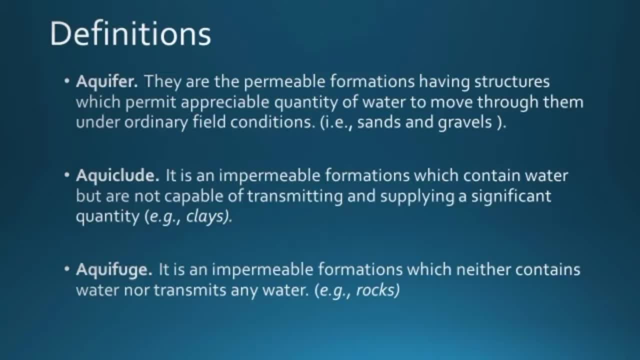 some definitions, aquifer. they are the permeable formations having structures which permit appreciable quantity of water to move through them under ordinary field conditions. The examples are sands and gravels. that is, they are permeable formations. Permeable means they allow water to run through it. Water will be very easily passing through those. 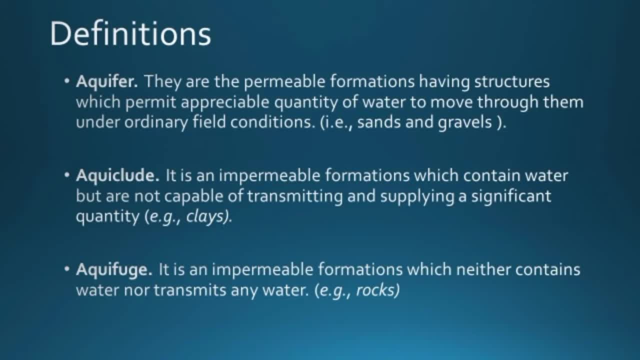 formations. ok, The examples are enough for understanding: sands and gravels. Next type of formation is aquiclude and, like aquifer, these are impermeable formations. They contain water, but they are not capable of transmitting and supplying any quantity of water. Clay is the example, So by that example itself you can understand that clay. 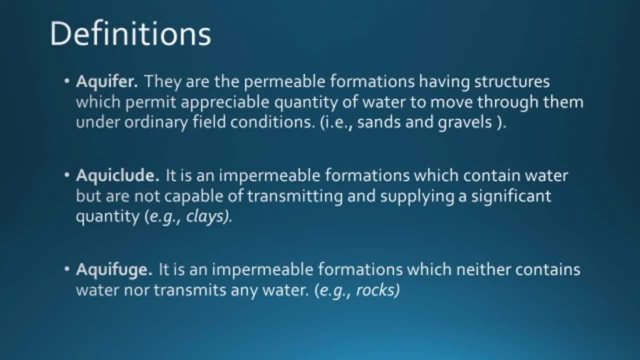 will be having a sufficient amount of water in inside it. But, unlike gravel or sand, we cannot collect water from clay. We cannot separate water and clay as you know it. So that is aquiclude. So the formation of our area below water table: we call that formation as aquiclude. 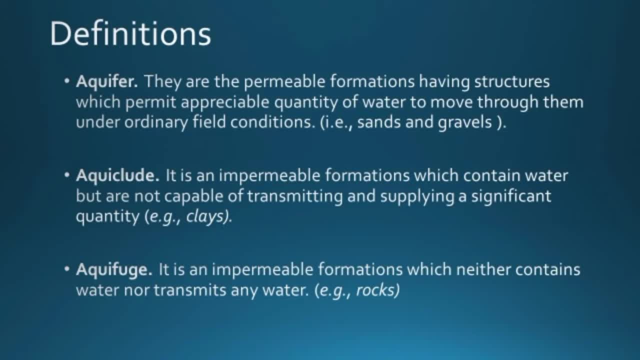 Third type of formation is aquifuge. It is also an impermeable formation which neither contains water nor transmits any. Example is rocks. So, as you can understand, if rock is the formation below our feet, underground rocks cannot contain any amount of water inside. 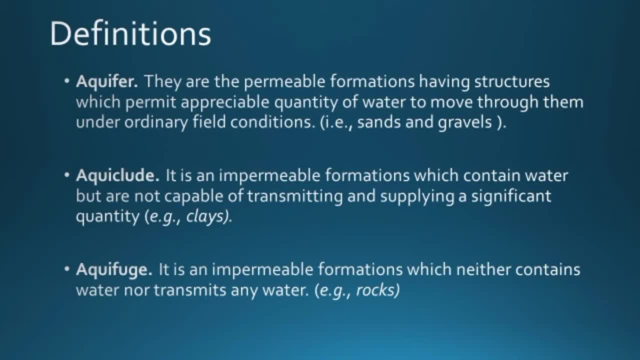 It is very hard. samples can be supplied or contain or pass through any water obviously, So they are called aquifuge. So from the definitions itself we can understand that to get ground water you need aquifer, So aquiclude and aquifuge. 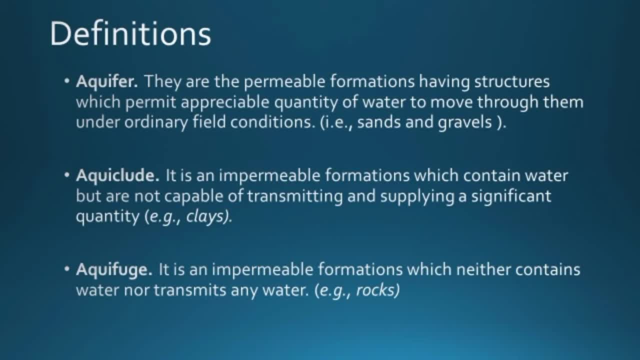 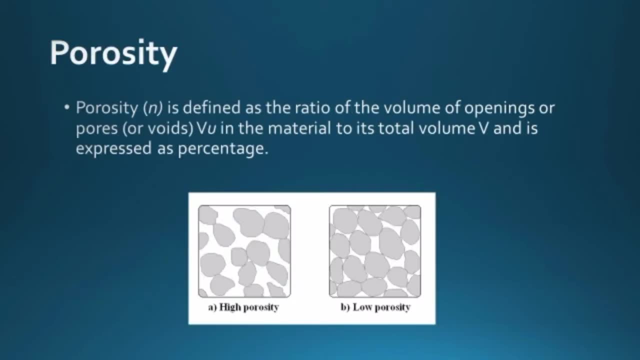 are not really useful or beneficiary when you are considering ground water. ok, So from now on, we will be concentrating on aquifers only. Before getting in to aquifers in detail, we should know three parameters to calculate a cliff. 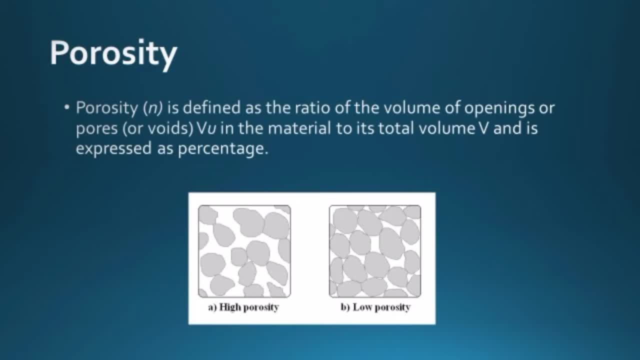 and assess the performance of groundwater supply from an aquifer. First one is porosity. Porosity is a very common term used in geotechnical engineering and many other engineering fields. Porosity is defined as the ratio of volume of openings or pores, commonly known as voids. 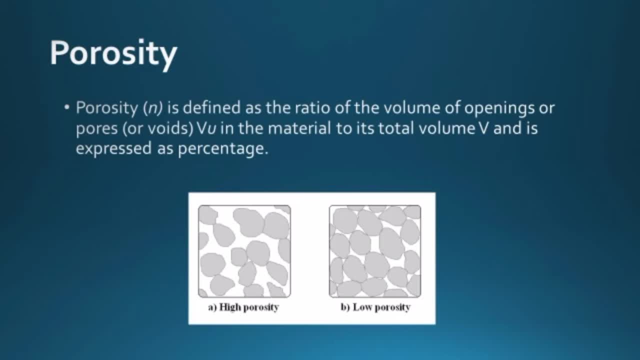 in the material. in our case, the material is soil to its total volume V, and is expressed as percentage. If you take a soil sample, there will be soil particles in it and there will be pore spaces, that is, vacant spaces where water can be occupied or air can be occupied. 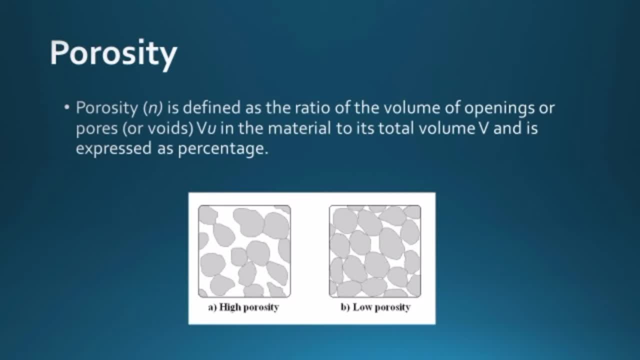 These pore spaces are called as voids, And porosity is just the ratio of that volume of voids to total volume, expressed in percentage. So, as the picture depicts, if there are more openings or pore spaces or voids, it is called as high porosity. 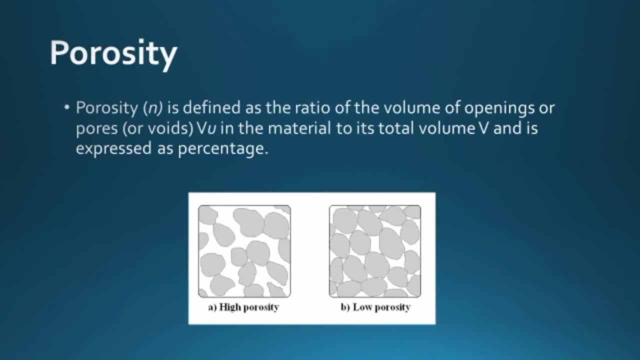 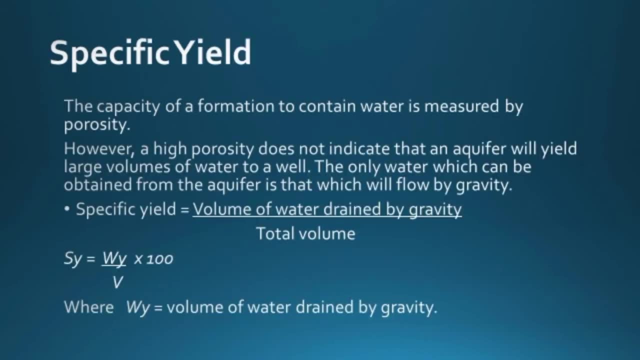 And if the soil particles are packed very closely and thus voids are very less, it is called low porosity. Next one is specific yield. As we know, yield is the ability of supplying water. It may be reservoir, it may be pond, it may be well. 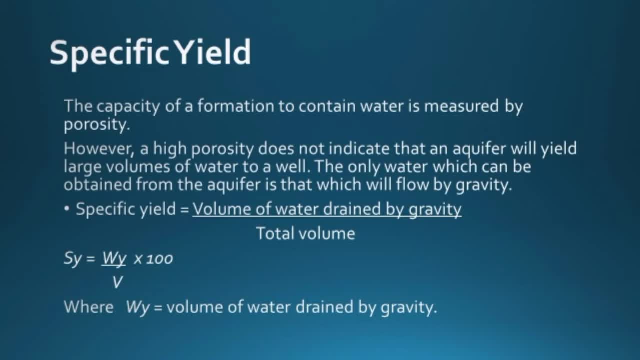 In this case it is aquifer or formations, And specific yield is volume of water drained by gravity divided by total volume S? y. specific yield is W? y divided by V into 100.. The concept behind specific yield is: with porosity you will get the maximum amount of water. 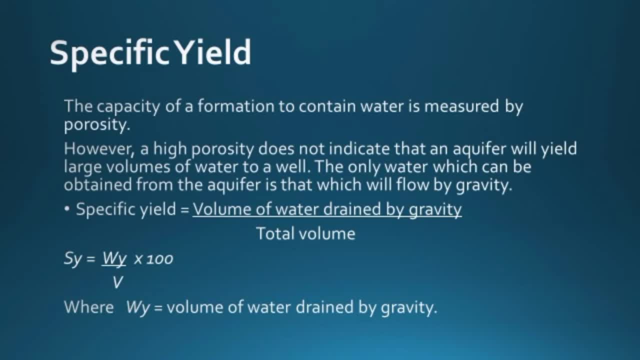 that is capacity of water that can be contained in a formation. But, as we said in the case of clay, the capacity by itself cannot guarantee the supply of water. By containing water will not guarantee that will supply, as we said in the clay matter. 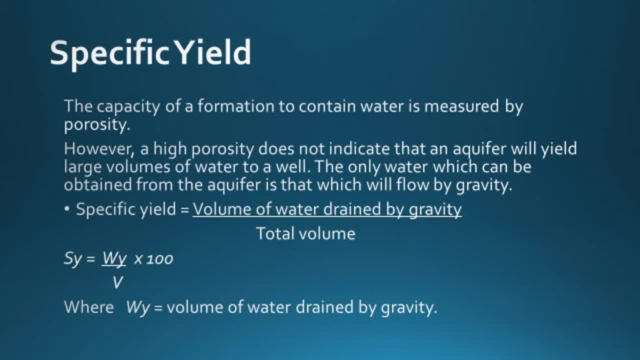 Clay have a considerable amount of water in it. it contains water but it does not yield any water. So specific yield is a measure to indicate the supplying characteristic or yielding characteristic of formation, That is, volume of water drained by gravity, that can be drained by gravity divided by total volume of water. 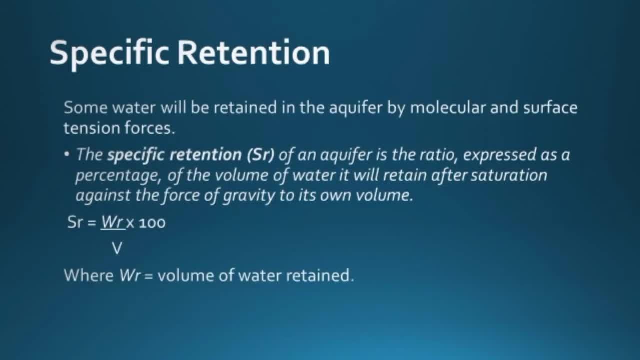 Next one is specific retention. Specific yield and retention is complementary terms. So if yield is the ability to supply water, specific retention is how much water is retained without supplying by gravity, The amount of remaining water after gravity supplying. So some water will be retained in the aquifer by molecular and surface tension forces. 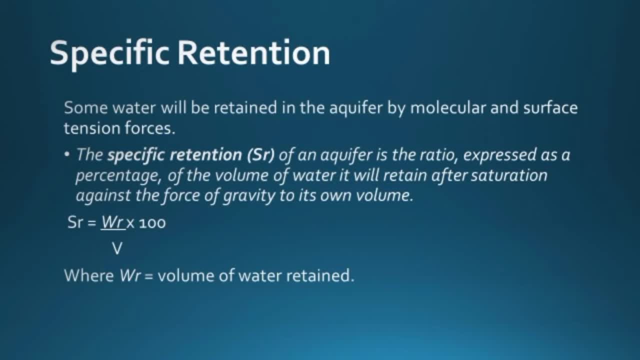 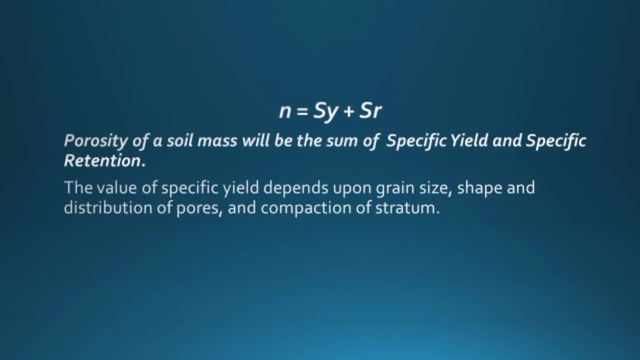 S? r is the ratio expressed as percentage of the volume of water it will retain after saturation against the forces of gravity to its own volume. W r by V into 100, where W? r is volume of water retained. And this is the relation between these three parameters. 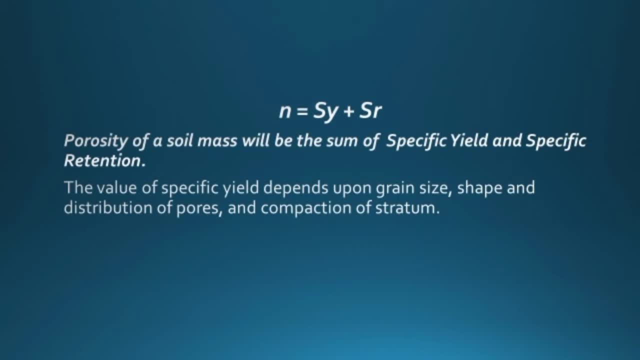 Porosity will be equal to sum of specific yield and specific retention, Because in a saturated formation there will not be any air particles inside the pores, So the total voids will be filled with water only. So the water yield by gravity and the water retained after gravity yield will be the total void space. 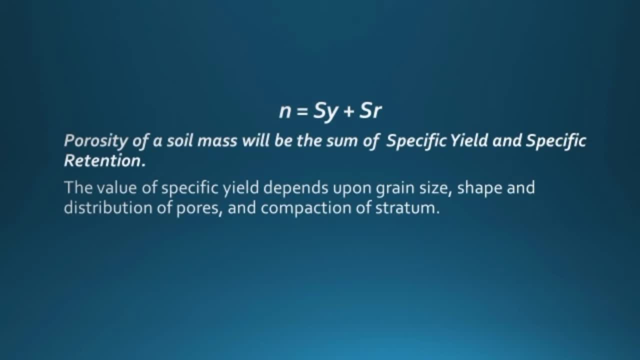 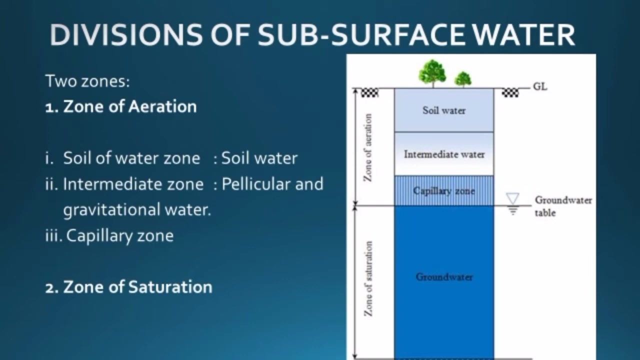 So N is equal to S y plus S? r. The value of specific yield depends on grain size, shape and distribution of pores and compaction of strata. Next one: divisions of subsurface water. How do we divide the subsurface water, the water beneath our feet? 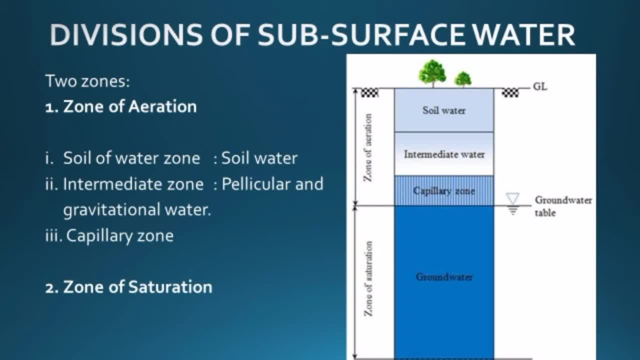 There are two zones primarily: Zone of aeration that is above water table, And zone of saturation. that is our main concern with the aquifers. Zone of saturation, which is below water table, And zone of aeration, is further divided into three. 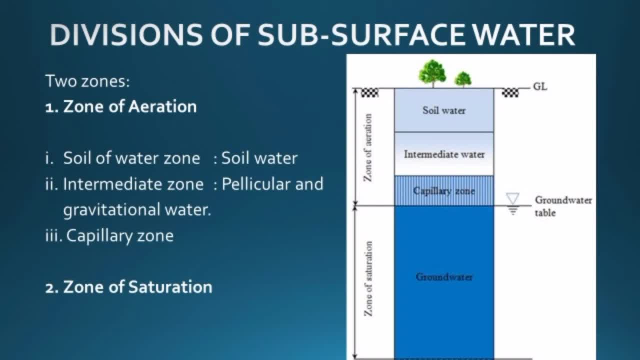 Soil water, intermediate zone water and capillary zone water. So, as you can see, these particular portions will be concerned with irrigation water, or root zone water as we call it, And the saturation zone will be concerned with our formations and aquifers. So the diagram is important. you need to know this diagram. 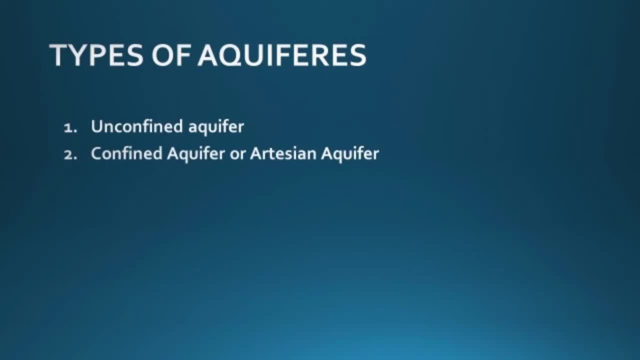 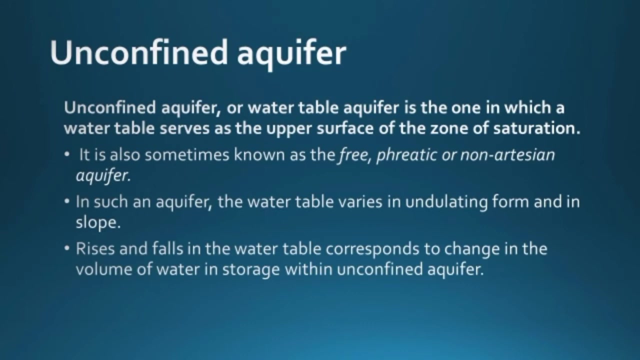 So we are getting into aquifers in details. There are two types of aquifers. First one unconfined aquifer and second, one confined or artesian aquifer. Unconfined aquifer or water table aquifer is the one in which a water table serves as the upper surface of zone of saturation. 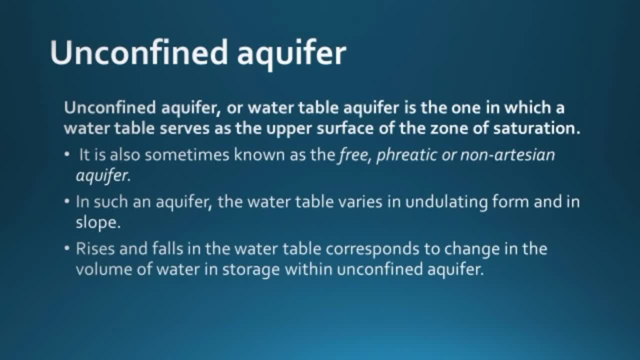 It is as simple as that. The upper portion of, or upper layer of, unconfined aquifer will be our water table. So obviously, unconfined aquifer is the most common type of aquifer we see all around us. It is sometimes also called as free phreatic or non-artesian aquifer. 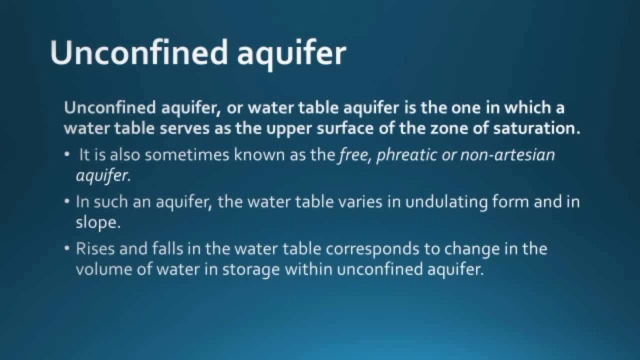 In these aquifers the water table varies in undulating form and in slope. Sometimes there will be rising slope, there will be sometimes falling slope. there will be undulations. These undulations and slope risings will be based on the storage of water in these aquifers. 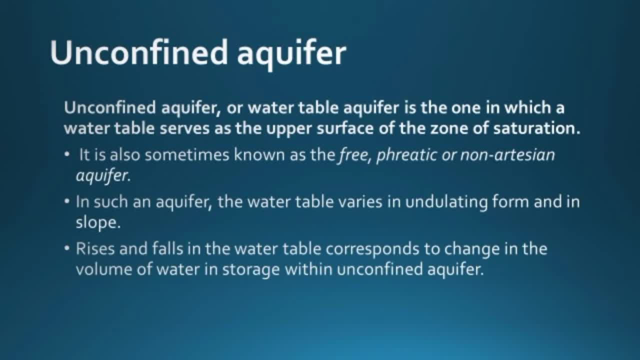 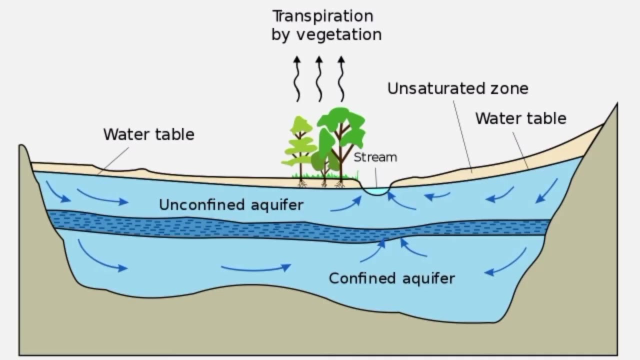 So these are just formations, but they are not unconfined. Unconfined means there is nothing to confine them, that is, to pressure them. There is just a layer of gravel with top layer as water table. So, as you can see, this is unconfined aquifer. 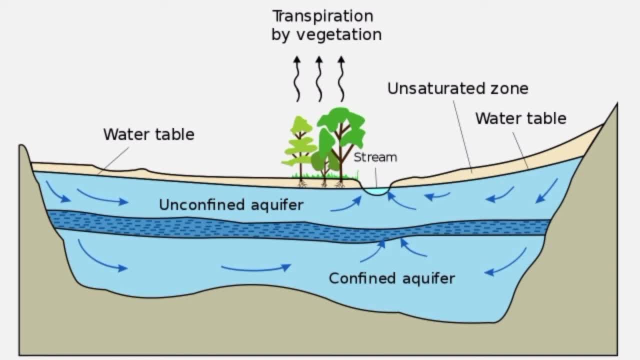 Water table is the upper layer. There will be slopes and undulations, depending on the surface formations, And this unconfined aquifer will sometimes will be joining with streams, lakes, rivers, etc. As you can see in this image. So unconfined means there is no confinement or anything. 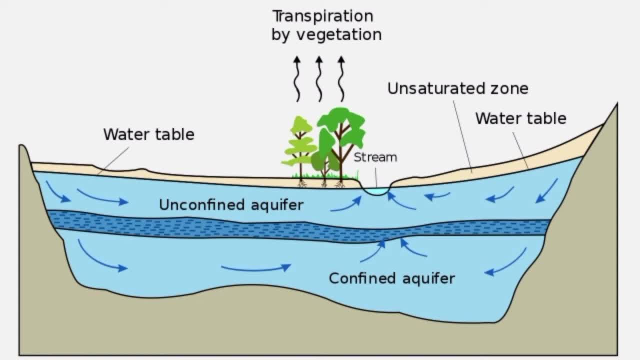 So, as you can see, below that unconfined aquifer there is confined aquifer, So confined aquifer. as the name indicates, there will be a confining layer of strata above this confined aquifer. Water table will not be the upper layer of confined aquifer. 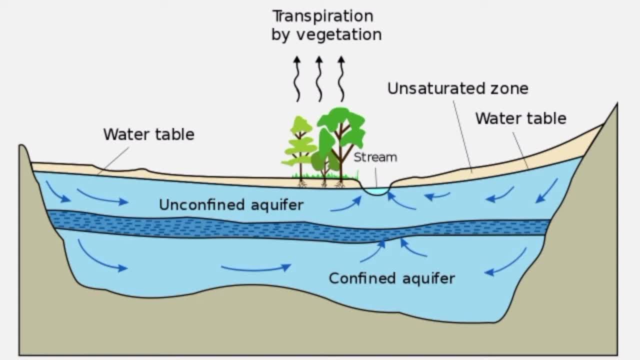 There will be a rock strata like this dark blue layer. It can be impermeable rocks or very hard clay, etc. It can be anything, but there will be a confining layer above the aquifer So that there will not be contact with water table and the aquifer. 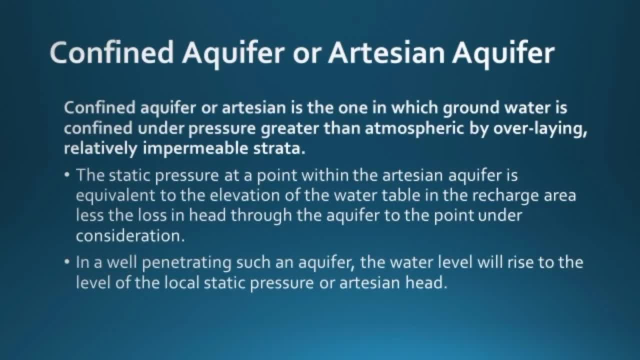 So confined or artesian aquifer is the one in which groundwater is confined under pressure greater than atmospheric by overlaying relatively impermeable strata. It can be rocks, hard clay, etc. The static pressure at a point within the artesian aquifer is equivalent to the elevation of water table in the recharge area, less the loss in head through the aquifer to the point under consideration. 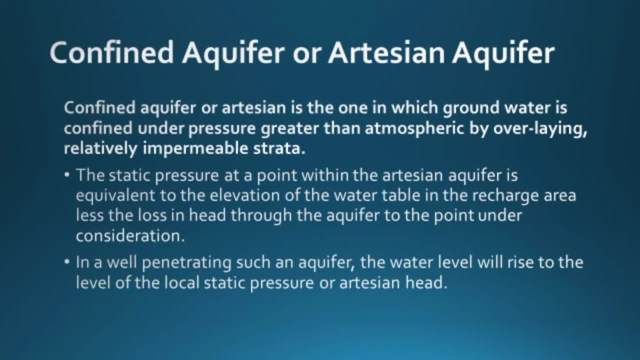 So to have water in an aquifer, in confined or unconfined aquifer, you need to get rainwater. So in case of confined aquifer, you will be having a recharge area which is open to atmosphere and through that recharge area, 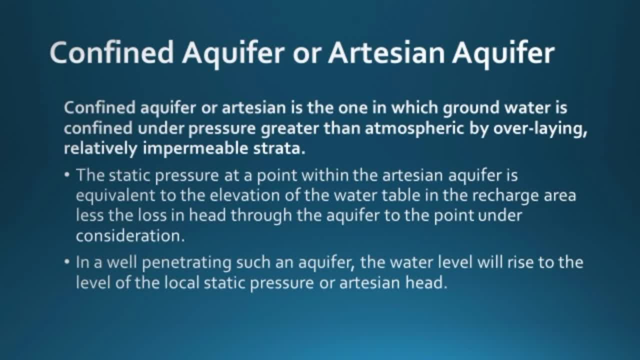 rainwater will be getting into this confined aquifer And static pressure at a point in the artesian aquifer will be equivalent to elevation of that recharge area minus the loss in head through the aquifer to the point under consideration. If a well is constructed to penetrate such an confined aquifer, 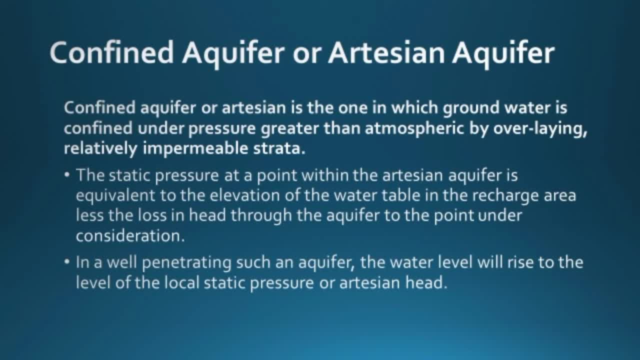 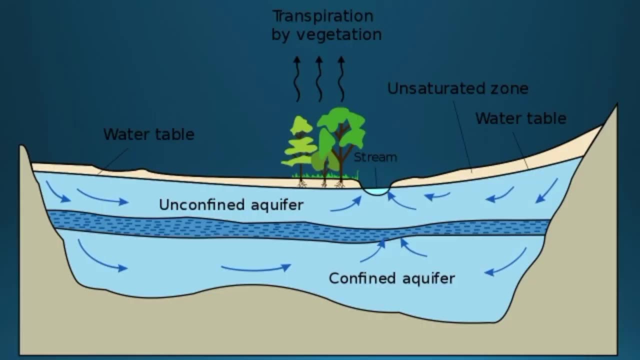 the water level will rise to the level of local static pressure or artesian head. Sometimes it may be above our ground level and this condition is called as flow wells. We will get to it shortly. So this is confined aquifer with an impermeable strata or semi-impermeable strata above it. 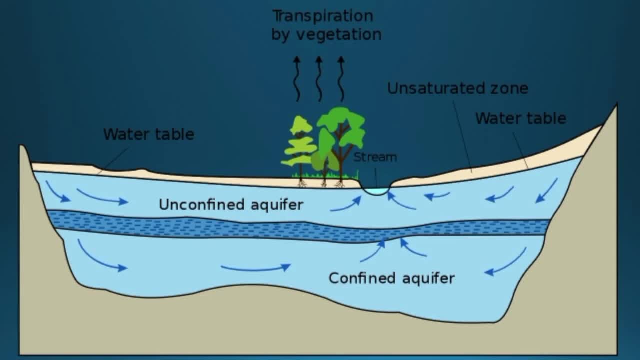 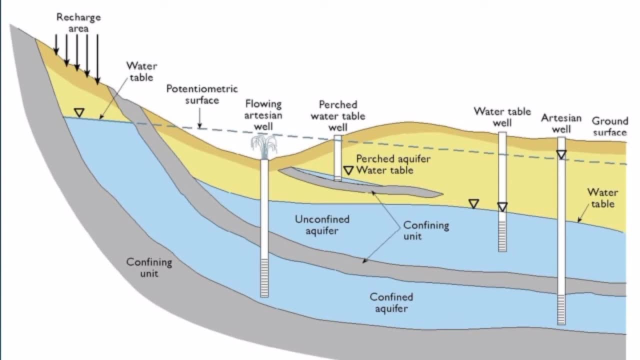 There will be a recharge area for any confined aquifer. It is just that we have not shown it in this image. See, in this image we have recharge area. Look in the leftmost side. through the recharge area, water will be getting inside and there will be a permeable strata over it. 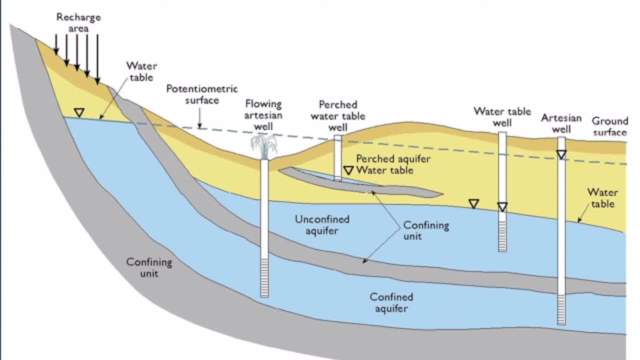 And the dotted line at the top part that slopes descendingly indicates the static pressure we have just talked about. Initially it will be the elevation of our recharge area and then it gradually decreases with the static pressure. with respect to pressure difference between the confinement and the aquifer: 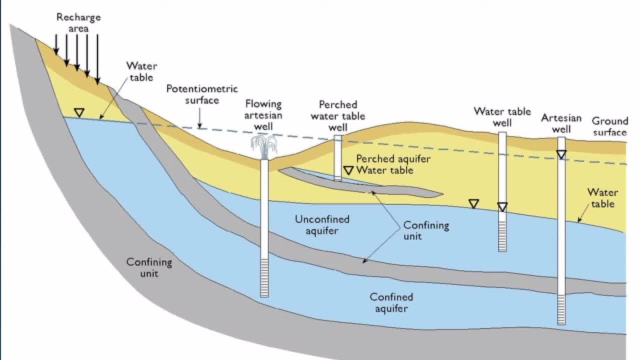 So in this image also we have unconfined aquifer with water table, undulating water table as a straight line separating between yellow and blue parts. So unconfined aquifer and confined aquifer. So normally when we construct a well into ground, 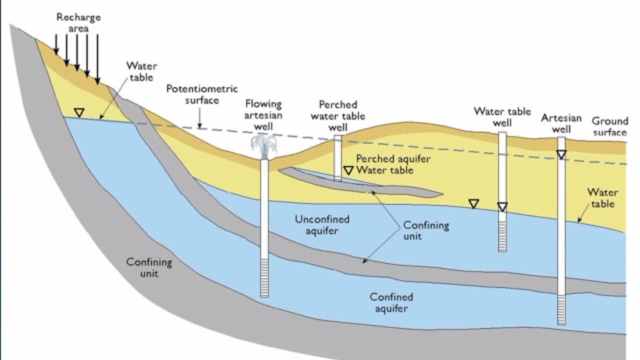 it is getting water from unconfined aquifer, So that well is known as unconfined aquifer well or water table well. It is called water table well because the water level in that well will be equal to water table in that area. 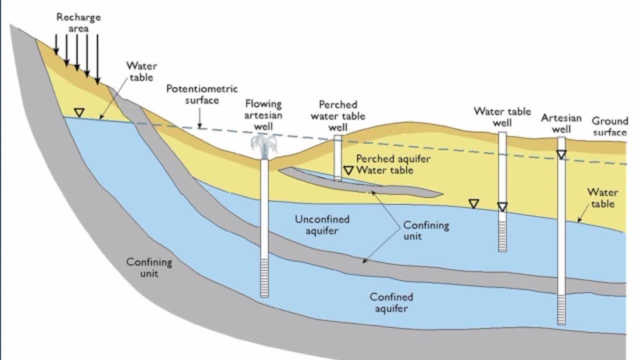 As shown in the figure. But if you construct a well penetrating that impermeable strata to a confined aquifer, the water level in that well will be that dotted line instead of water table. So, as you can see in the image, water table is lower than that static pressure. 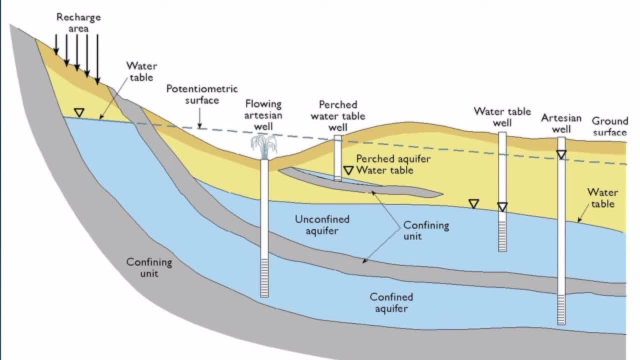 dotted line, static pressure, or piezometric level, we call it, or potentiometric surface, we call it. So the point is if you are getting a well penetrating that impermeable strata, confining strata into a confined aquifer and getting water from confined aquifer. 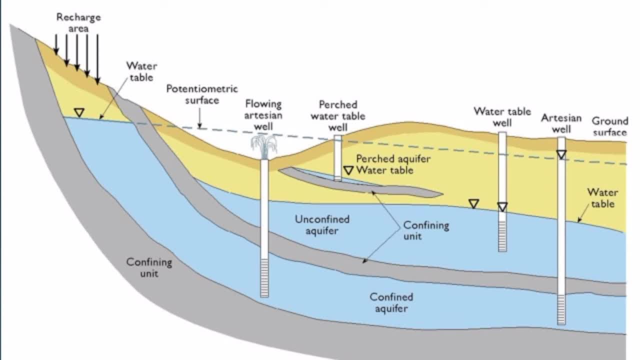 you will be getting water level with respect to piezometric level or static level. And what happens? if suppose that piezometric level is more than the height of ground, that in that well shown in the left side, flowing artesian well, In that the dotted line is static pressure at that point. 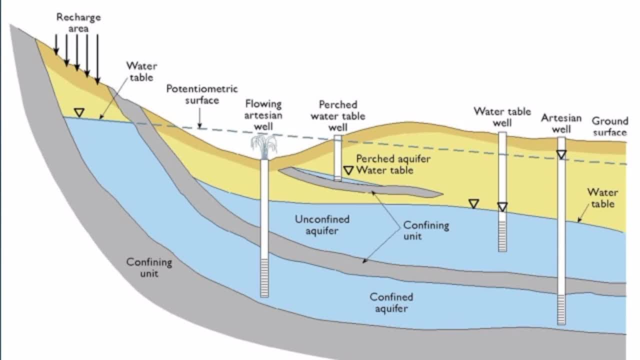 The ground level is below that static pressure. So if you get to construct a well into confined aquifer in that area, the water will be always flowing out, pumping like a pump, So that flowing water well is known as flow well or flowing artesian well. 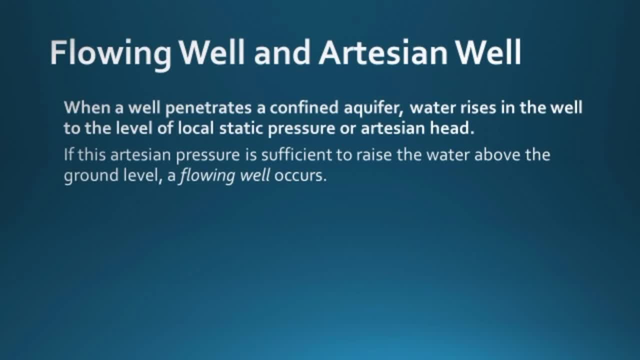 When a well penetrates a confined aquifer, water rises in the well to the level of local static pressure or artesian head. If this artesian pressure or head is sufficient to raise the water above ground level, a flowing well occurs That is flowing well. 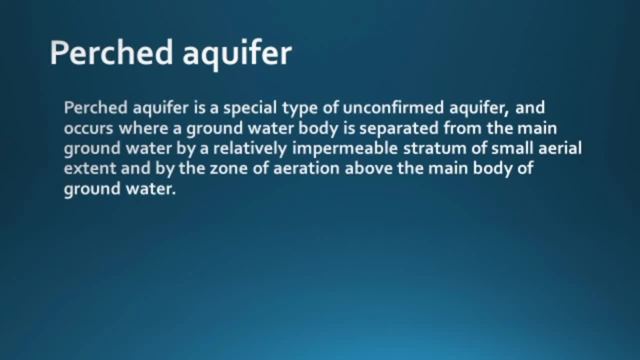 Next one, perched aquifer. It is a special type of unconfined aquifer and occurs where ground water body is separated from the main ground water by a relatively impermeable strata of small aerial extension and by the zone of aeration. 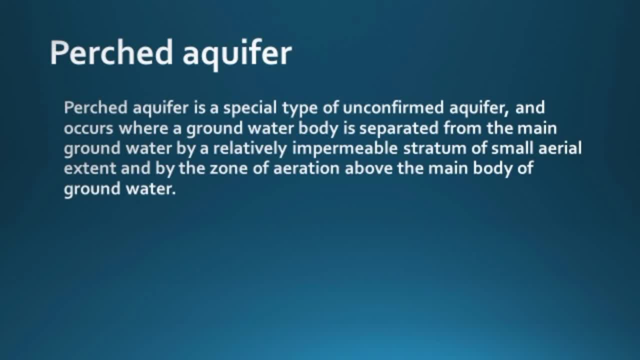 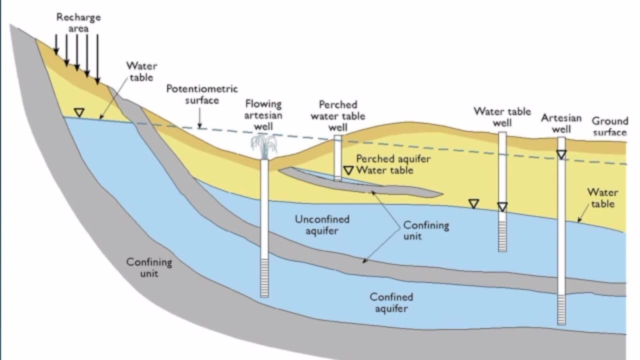 above the main body of ground water. It is like some water is kept aside, with a small vessel. See, at the center there is a confinement and there will be a portion of water in that formation and that will be above water table. So that is perched aquifer. 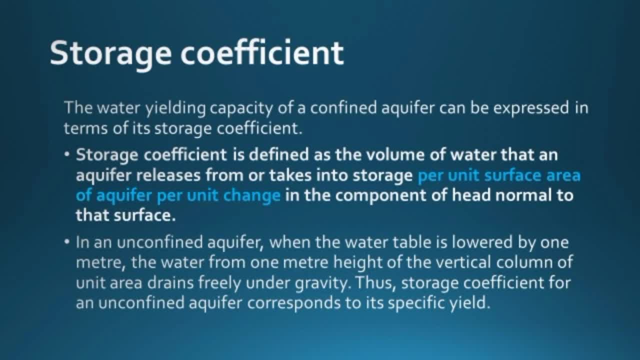 So, as the last portion of this video, we have three more parameters to define. on First one, storage coefficient. It is defined as the volume of water that an aquifer releases from or takes into storage per unit. surface area of aquifer per unit. change in the compound of head normal to that surface. 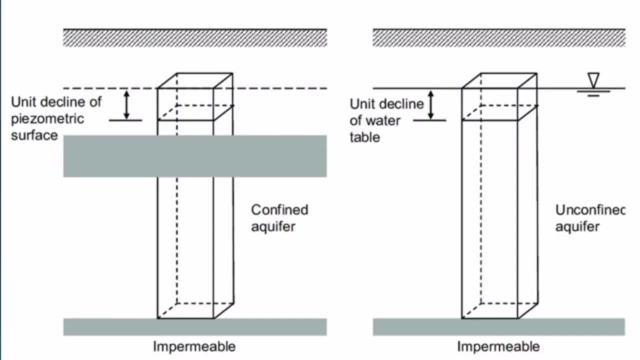 No need to get confused, it is very simple. Consider this much area, Consider the right one, which is of unconfined aquifer. There is no confinement, So this is an imaginary prism of volume considered in an unconfined aquifer with unit cross section. 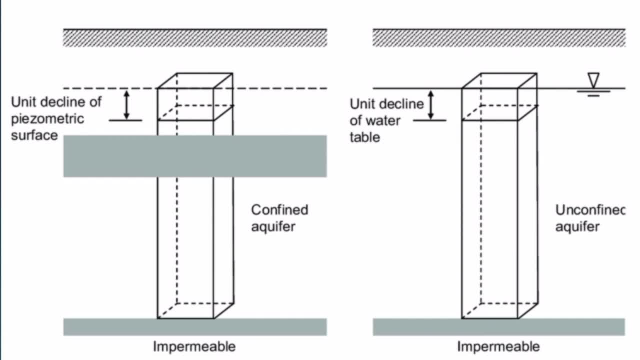 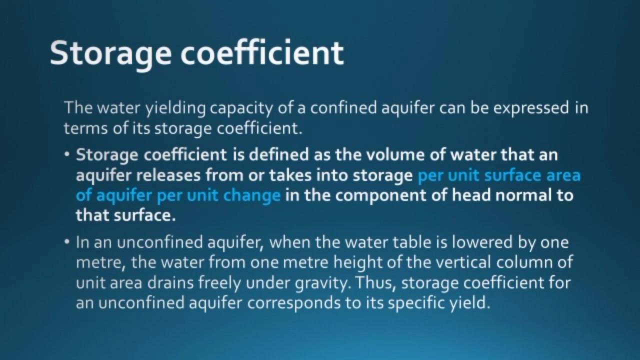 So consider that area and how much water will it take to increase or decrease the water table of that particular area? only That volume of water that can be supplied or yielded is called as storage coefficient. It is simple as that. So the storage coefficient is water releases from or takes into storage per unit surface area, per unit change in the compound of head normal to that surface. 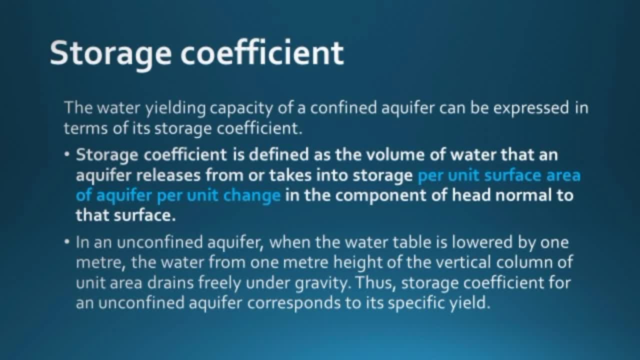 That is it In an unconfined aquifer. when the water table is lowered by one meter, the water from one meter height of vertical column of unit area drains freely under gravity. Thus storage coefficient for an unconfined aquifer corresponds to its specific yield. 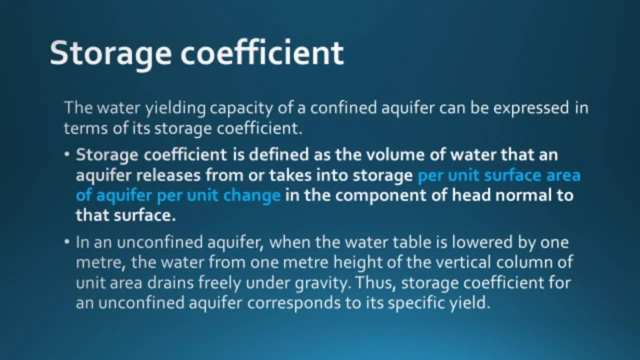 So when we are considering unconfined aquifer, this storage coefficient will be equal to specific yield that we have discussed previously, Because the only force getting into action in an unconfined aquifer for water supply will be the gravity force, which was used to find specific yield. 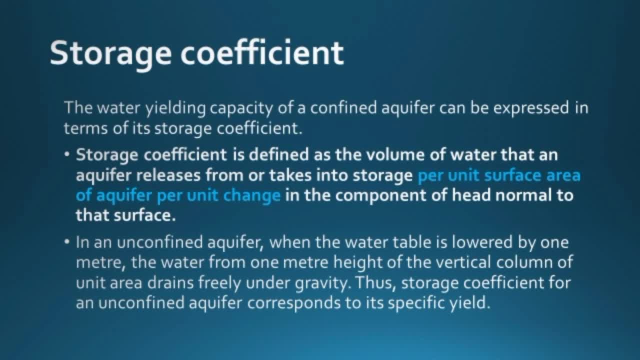 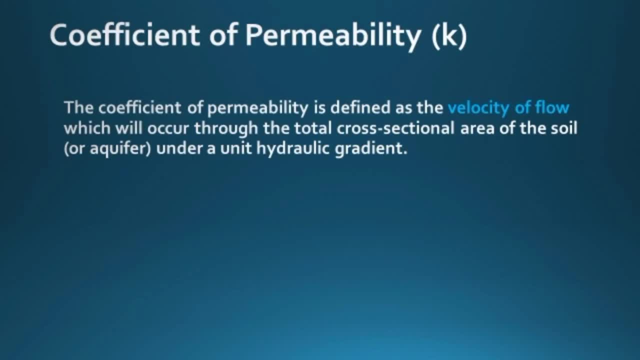 So storage coefficient is a term to study water yielding capacity of a confined or unconfined aquifer. Second one, coefficient of permeability. It is defined as the velocity of flow which will occur through the total cross sectional area of soil under a unit hydraulic gradient. 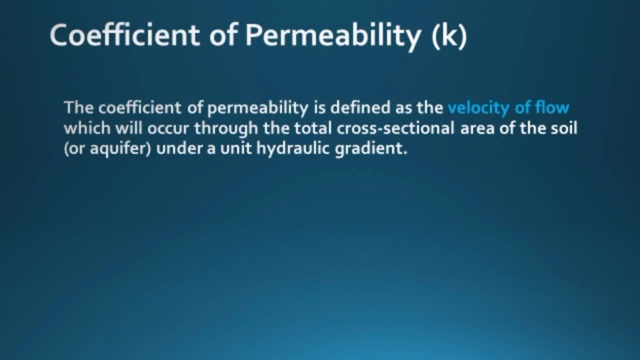 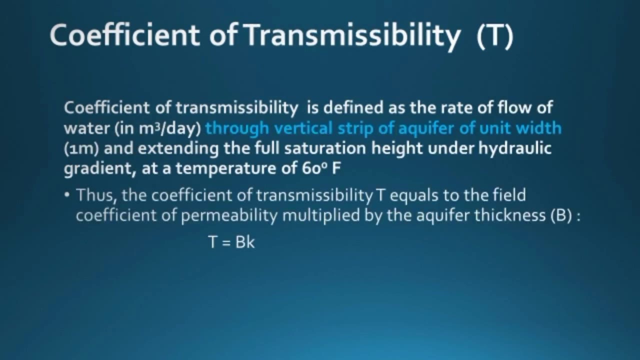 So, unlike storage coefficient, which was the volume of water that need to be supplied, it is velocity of flow through the total cross sectional area under unit hydraulic gradient, And the last one coefficient of transmissibility, or capital T. It is defined as the rate of flow of water or discharge in meter cube per day through the vertical strip of aquifer of unit width. 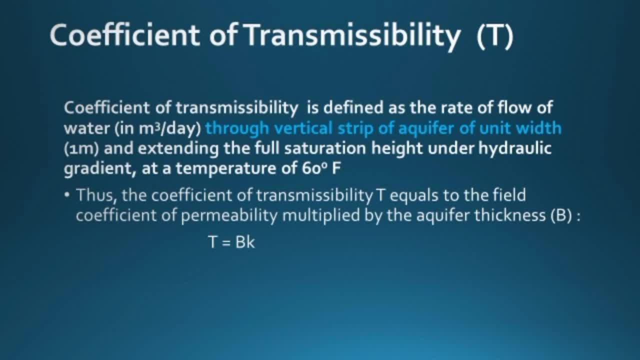 That is 1 meter, and extending the full saturation height under hydraulic gradient. It is taken at a temperature of 60 degree Fahrenheit And the coefficient of transmissibility, capital T, equal to permeability coefficient multiplied with aquifer thickness, That is capital B.